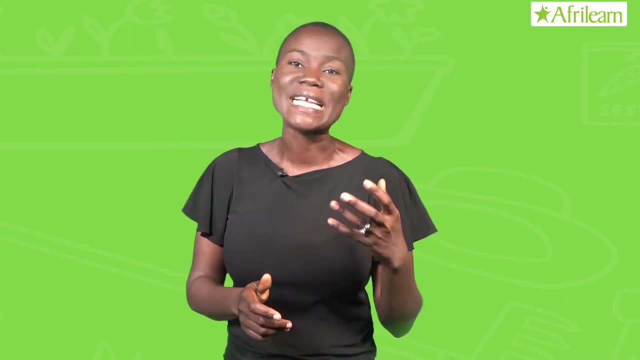 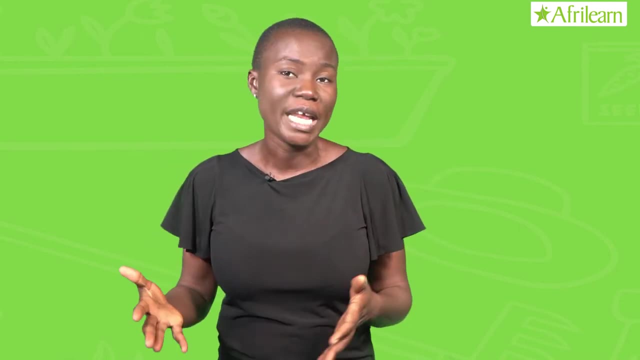 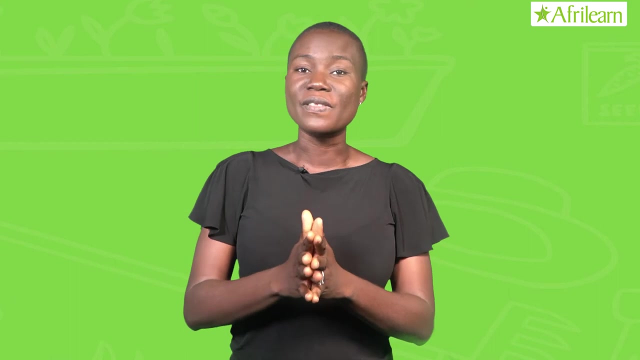 like burning, destroy the fertility of the soil by destroying its nutrients, the way burning destroys the nutrients in the pot of food. You can also liken overwashing vegetables to leaching and erosion of the soil. These factors, and more, affect nutrient availability in the soil, and we will be listing some of 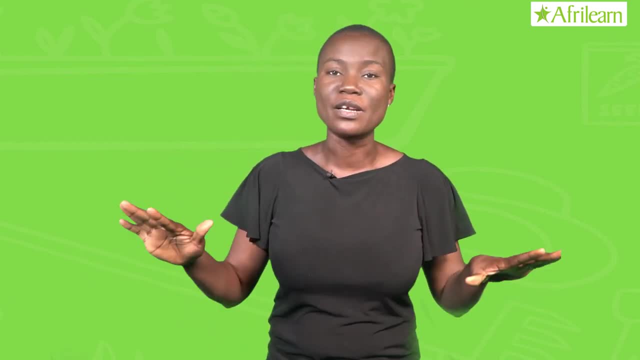 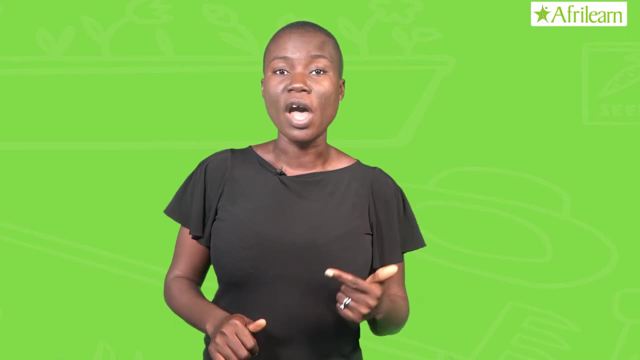 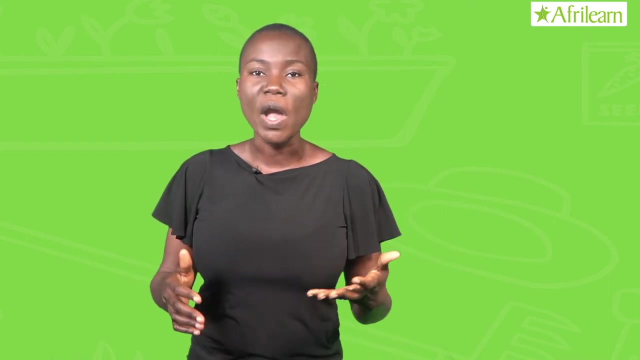 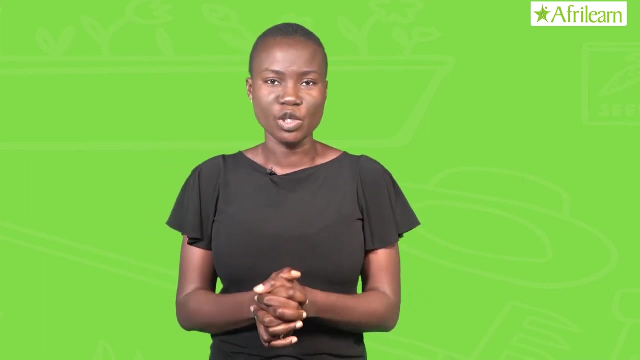 these factors. today, There are several factors that could affect the nutrient availability in the soil. Some of these factors are soil pH, consecration of other nutrients, leaching, crop removal, oxidation and reduction of organic material and the soil texture. These factors will most likely lead to the loss of soil nutrients. Earlier, we had already 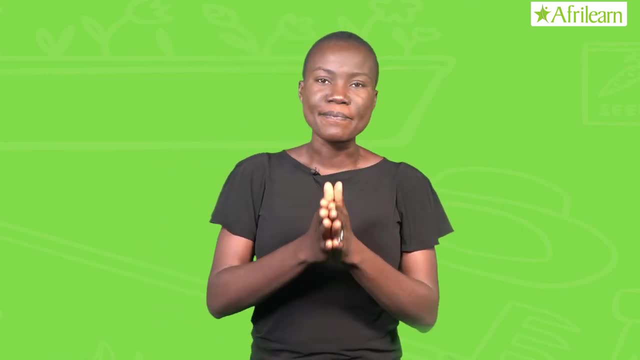 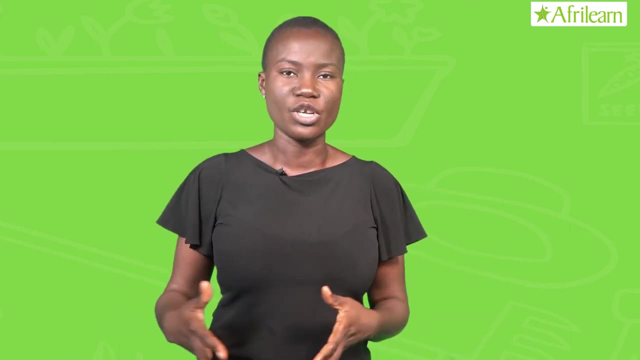 mentioned burning, erosion and leaching as factors that deplete the soil of nutrients. Soil nutrients can also be lost when the soil contains excess of other nutrients. With these we have come to the end of our lessons on farming practices. We hope you have enjoyed. them so far. 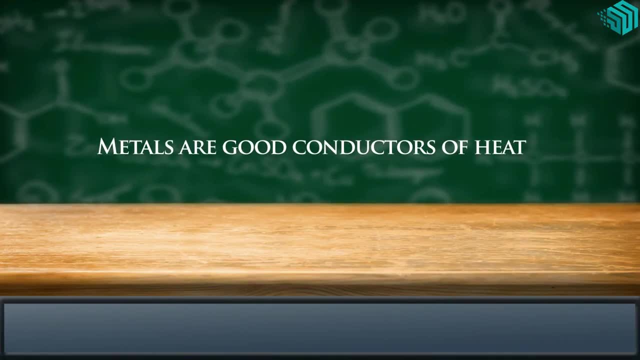 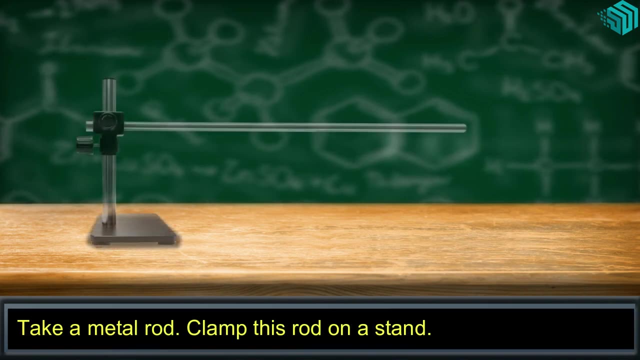 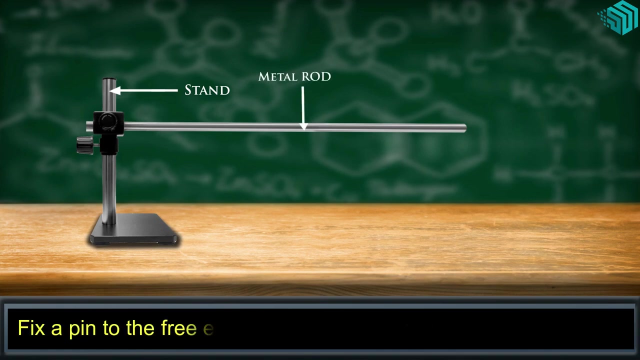 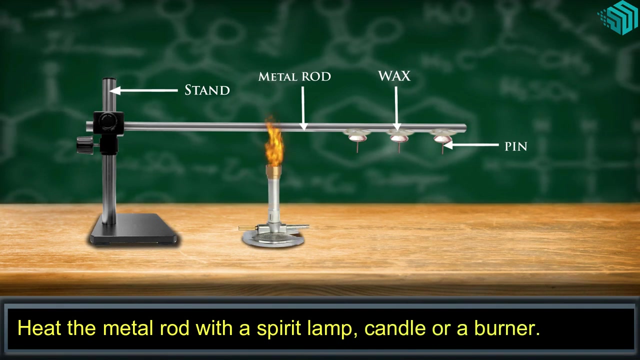 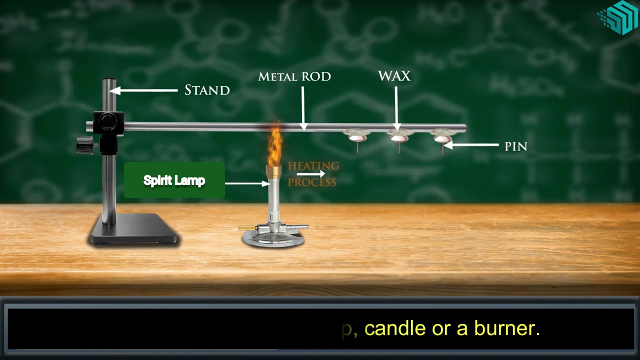 Metals are good conductors of heat. Let us learn this through an experiment. Take a metal rod. Clamp this rod on a stand. Fix a pin to the free end of the rod using wax. Heat the metal rod with a spirit lamp, candle or a burner near the place where it is clamped. 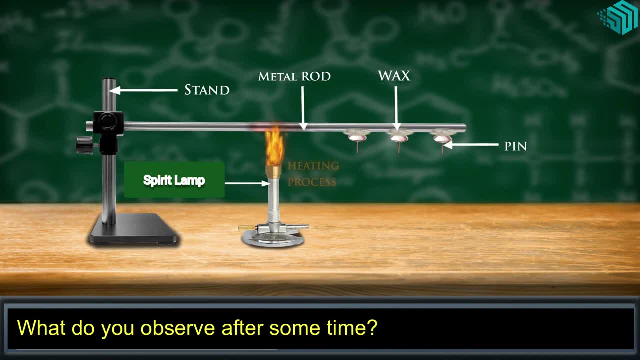 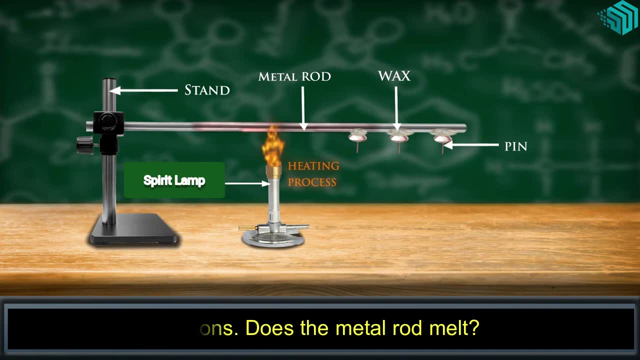 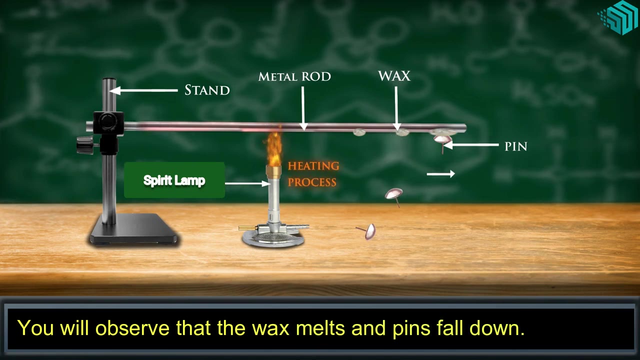 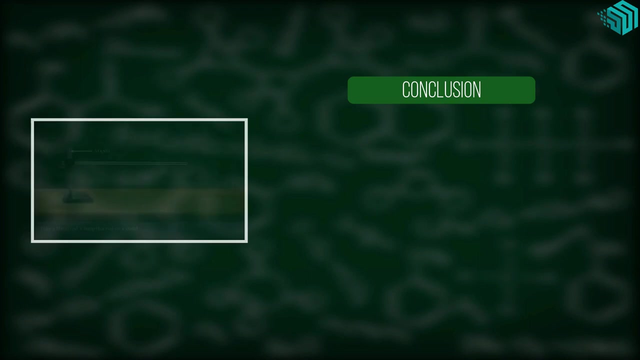 What do you observe after some time? Note your observations. Does the metal rod melt? You will observe that the wax melts and the pins fall down. So we get down to the conclusion that the activity shows that metals are good conductors of heat and have high melting points. Let us go to look at another example. This is another example. This time the metal rod was far from hot. A piece of metal is put together to form a solid metal. The metal rod does not melt. An another example shows that a piece of metal is not hot.